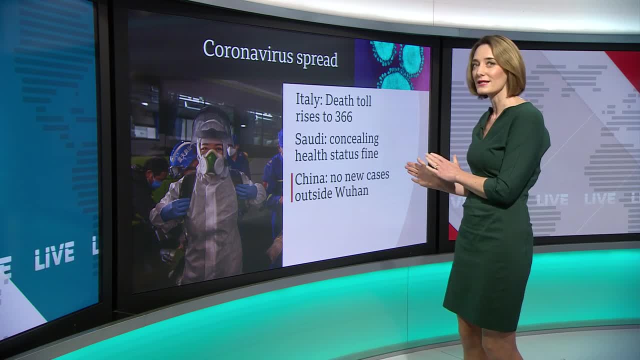 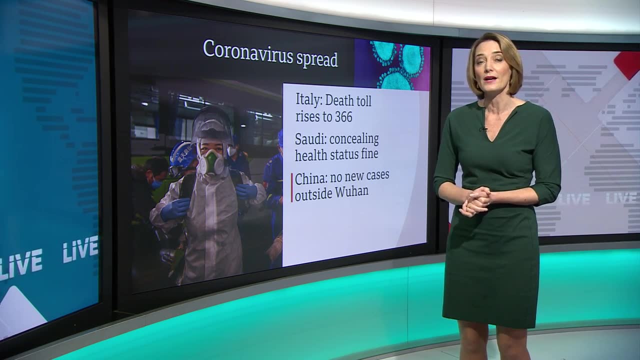 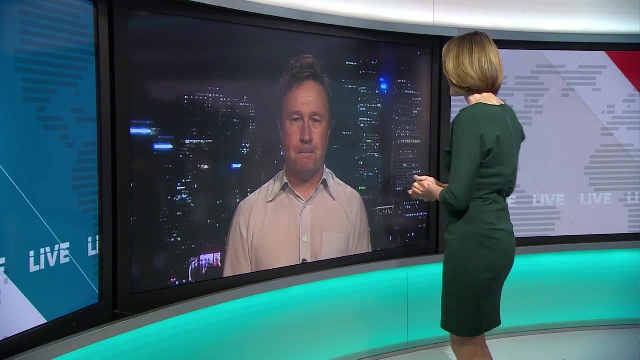 country. There is one glimmer of hope, though, in this battle against the virus. The Chinese province of Hubei has had no new cases outside the city of Wuhan for the second day running. So let's take you live to Beijing and speak to our correspondent, Stephen McDonald. Steve proof, then, that these 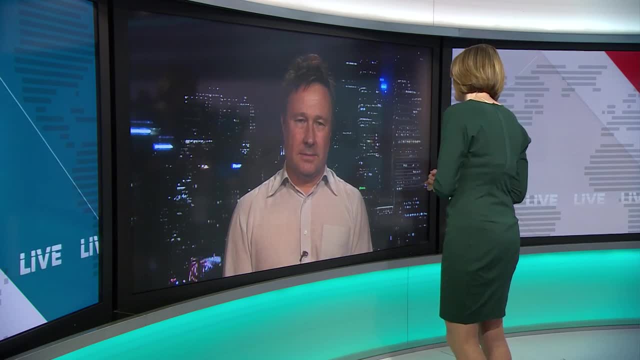 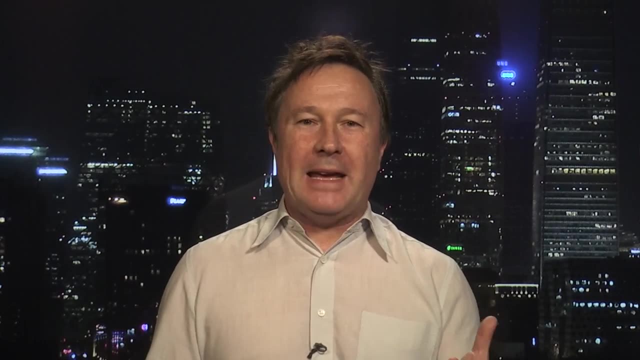 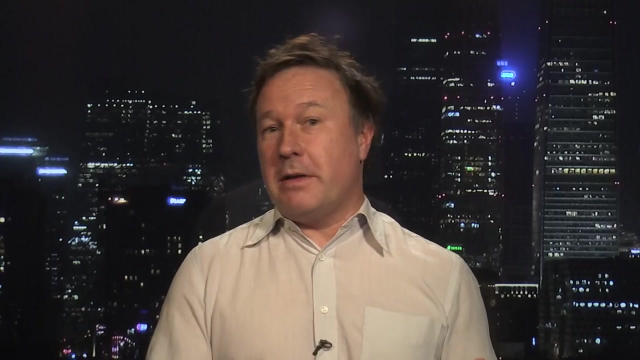 draconian measures implemented in China work. Yeah, we have sort of two very different pictures here, if you like. We've got the global panic on stock markets, with people talking about an international recession following the coronavirus spreading here and everywhere, And on the other hand, we have a situation in China where- well, 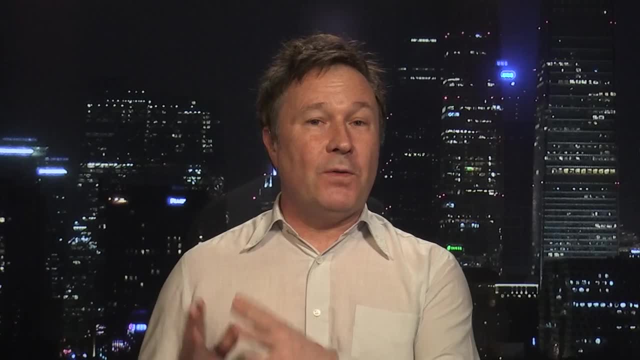 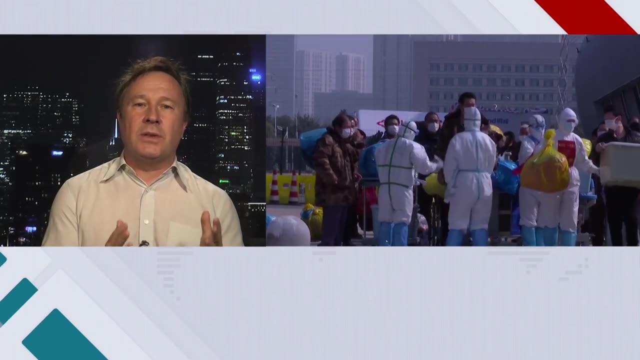 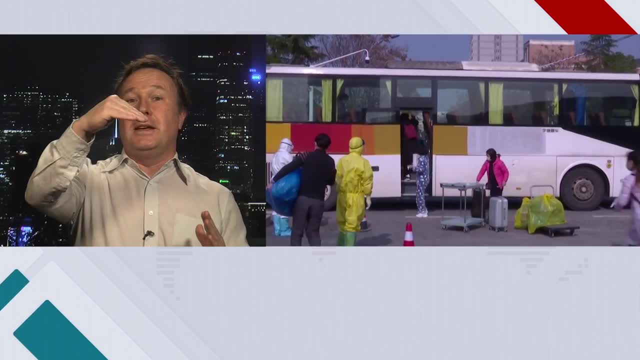 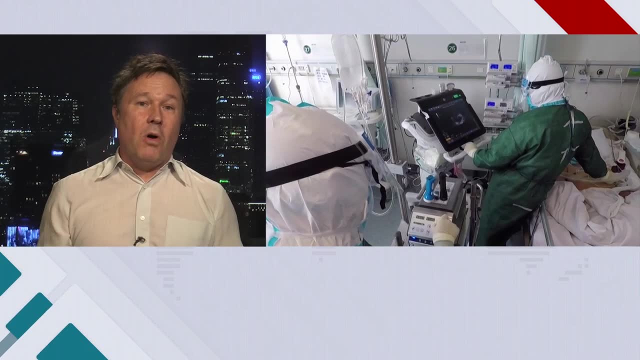 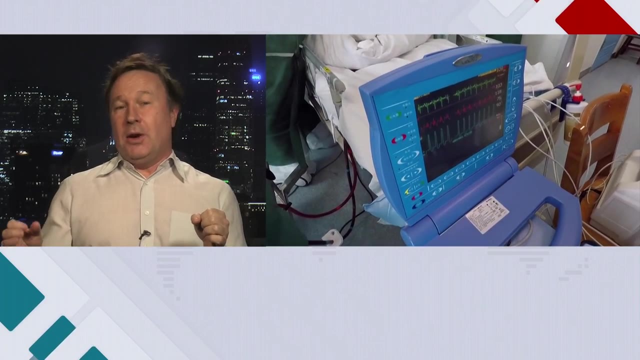 is that the problem has gone like this in Wuhan and sort of and is now coming down And you look at the picture in the rest of the China, it's even more optimistic. I mean, if you take that one city of Wuhan out of the picture and also people who are arriving in China from overseas, bringing the 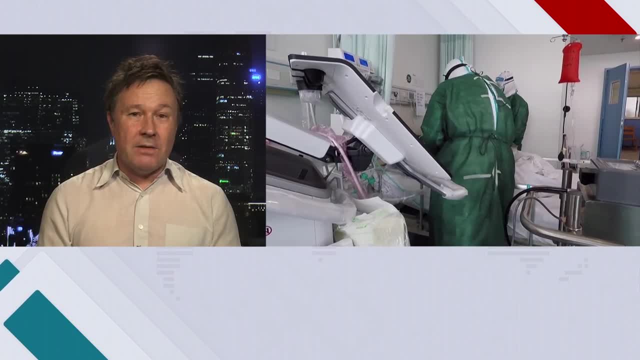 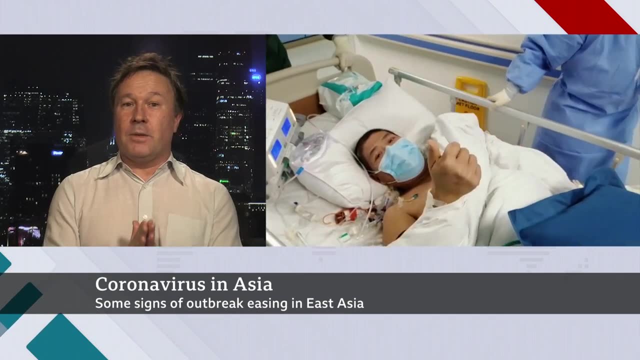 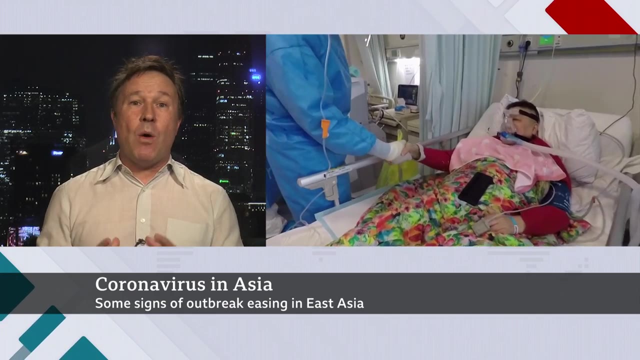 coronavirus with them. for the last four days in a row, we've had zero extra coronavirus infections. Now that would that would seem to suggest that the prop that these measures being put in place in China, quite strict measures restricting people's movements, are working. Also, you know, you look at South Korea. 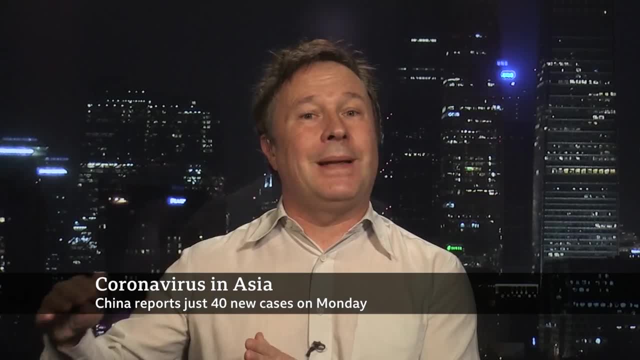 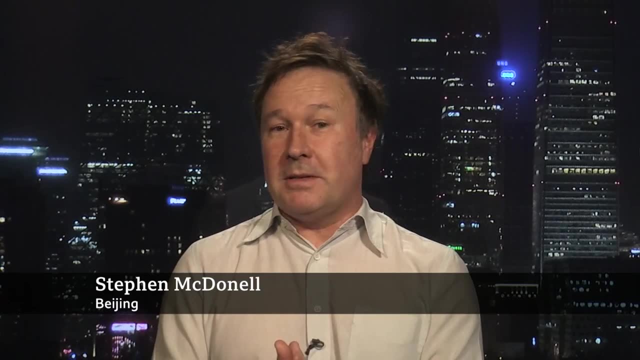 the situation for the moment does seem to be also plateauing there. Now people in other countries might take some hope from this, but that doesn't help them in the short term, Because elsewhere, you know, as the coronavirus hits economy after economy, there is going to be some pain, And when. 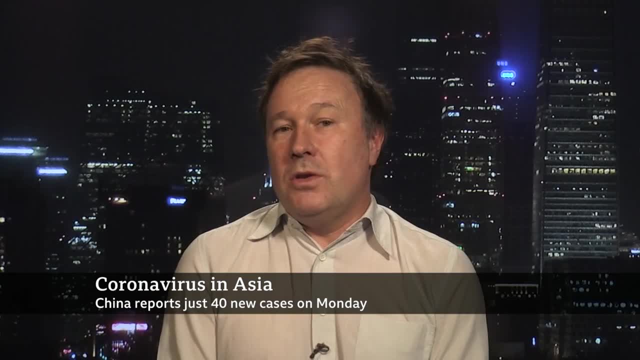 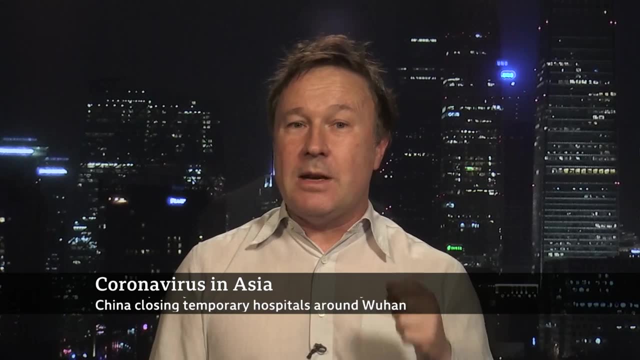 you look at the markets, you know, I think, the difference is those who are gambling, which is what it's all about. on the short term versus the long term, people can see there is going to be short term pain, Although eventually, you know, this problem will be sorted out. 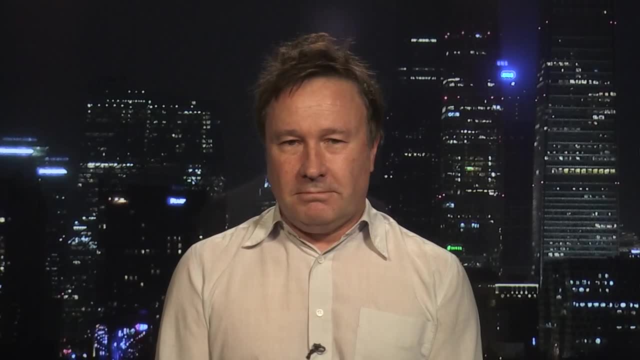 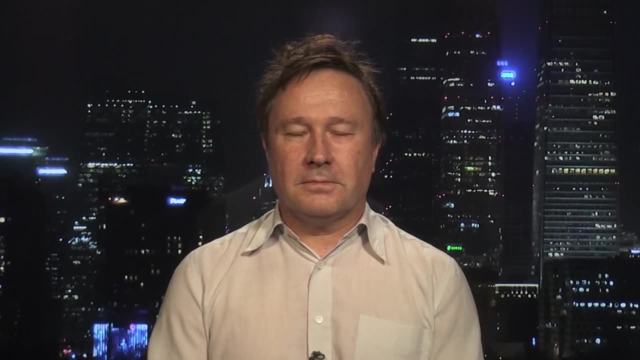 Steve, thanks so much for joining us. Steve McDonald, there, live for us in Beijing. Well, let's update you now on what is happening in Italy, because the government has said it will increase spending to offset the economic impact of COVID-19.. 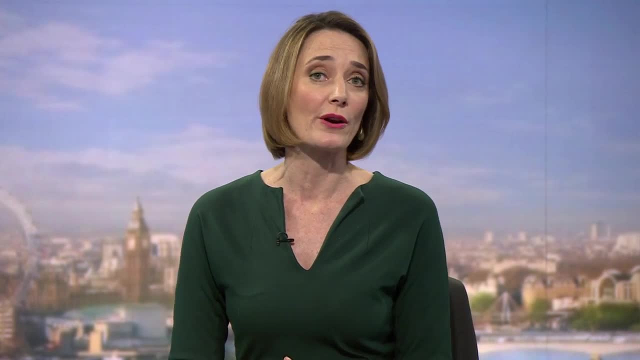 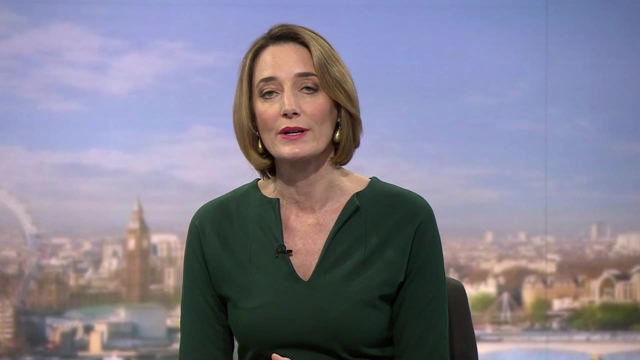 of the coronavirus and what the Prime Minister has described as shock therapy. that's, after the death toll from the virus shot up by 133 on Sunday, the total number of infections has also increased dramatically. strict measures have been introduced to reduce social interaction, especially in the northern regions, which 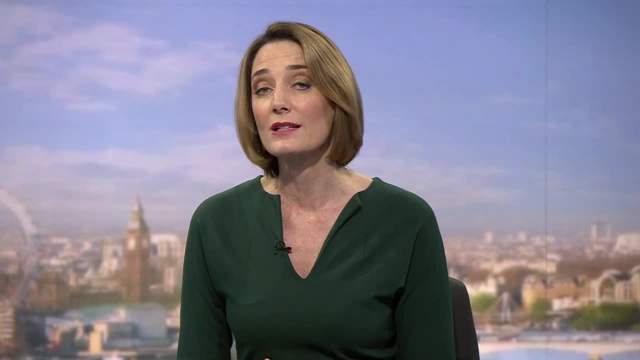 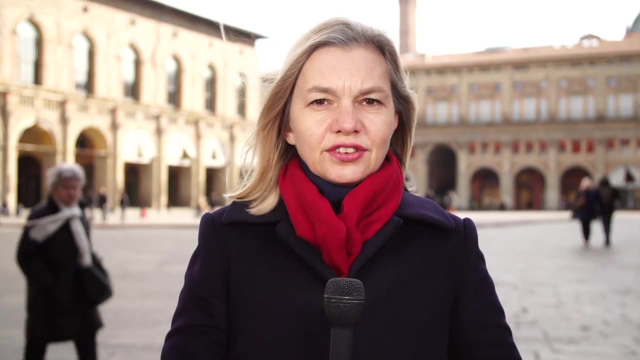 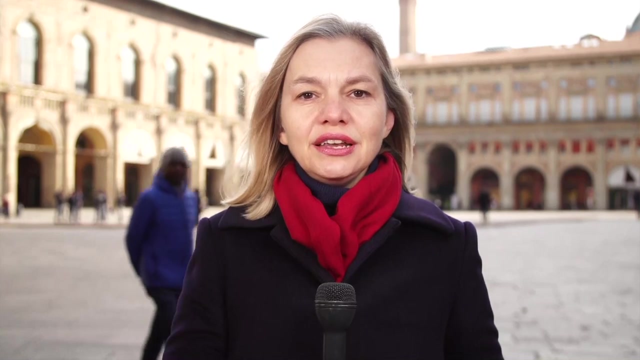 are the worst affected areas. for more on those measures, I've been speaking to our correspondent, Bethany Bell. she is in Bologna, which is just outside the affected area. we're guessing a few more details as to exactly what this partial lockdown means. we're told that people are not allowed to leave Lombardy or to 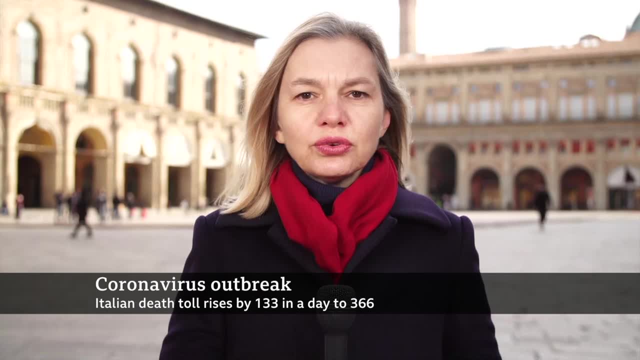 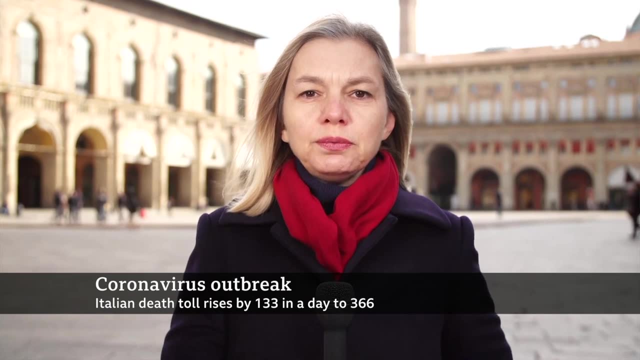 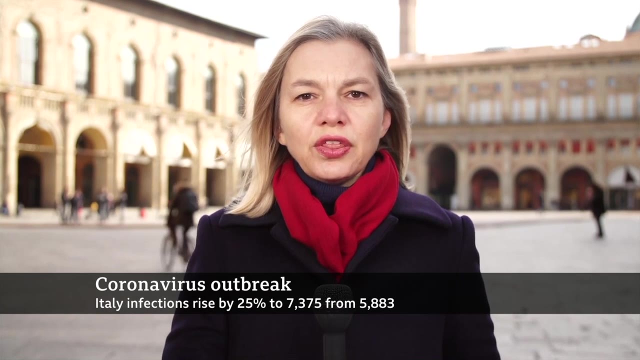 enter Lombardy unless they have very important essential work related reasons for doing so or emergency family reasons, and people will be checked if they try to leave airports or train stations and asked to give their justification for their movements, people also being encouraged to stay where they are. 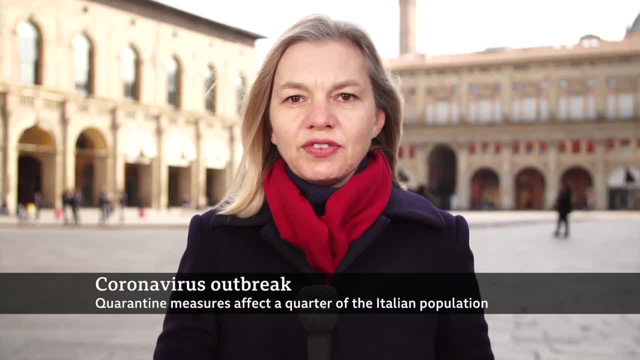 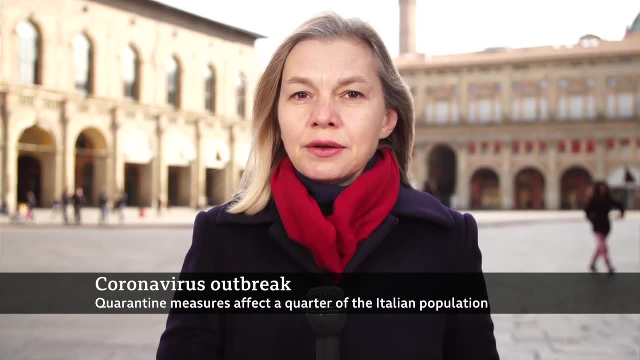 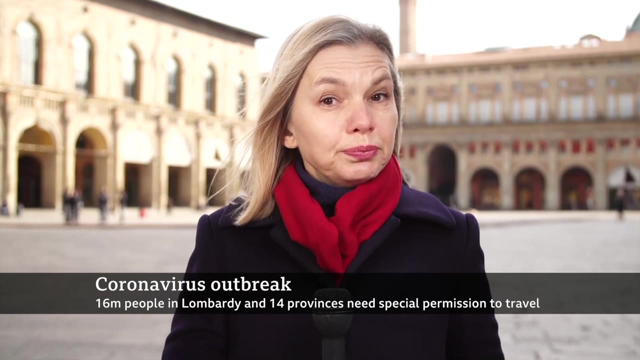 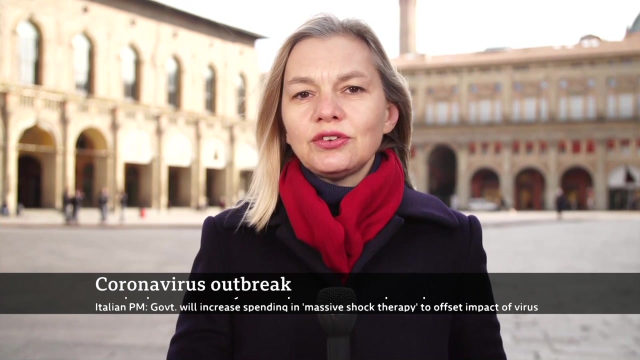 within those regions to try and prevent the spread of the disease. now also, we've seen lockdowns, as we heard in Venice. people here are getting very concerned about this on the impact of the economy and the. the actual governor of Veneto, where Venice is, has actually said that he believes that Venice, Padua and Treviso should not be. 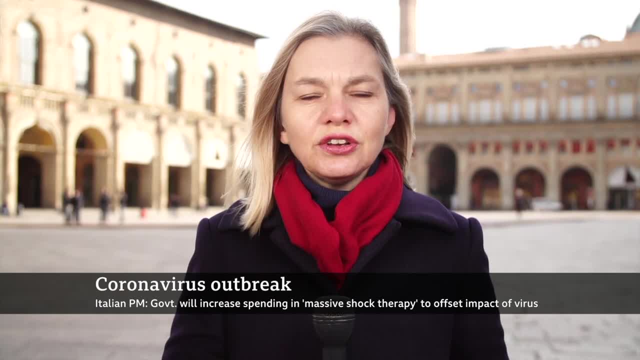 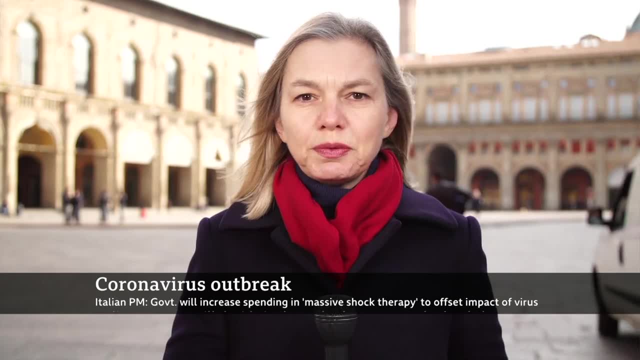 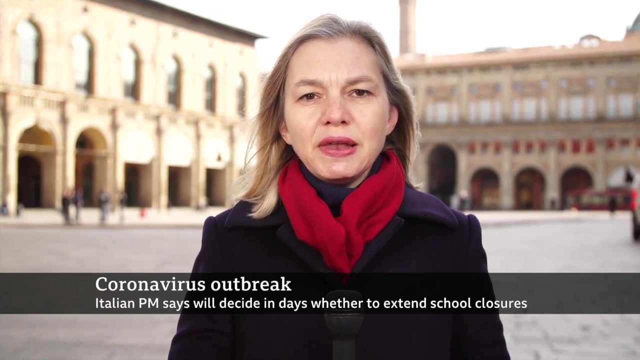 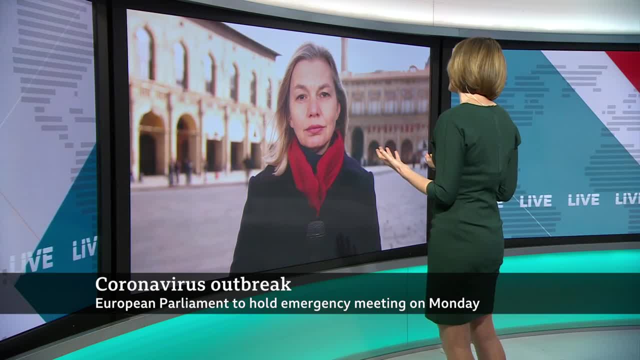 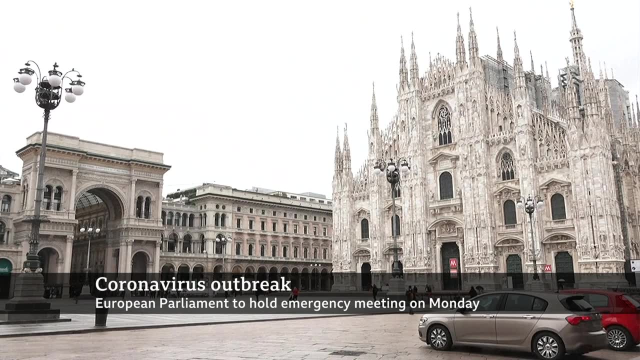 emergency. maybe the government has been phase two, slowly imposing these kind of strict measures, that we're waiting to see just how firmly and strictly the authorities will actually try and police these. Bethany, you're in Bologna, but we have some live pictures coming to us at the place. you were last week, right outside the Duomo, the Cathedral in Milan. 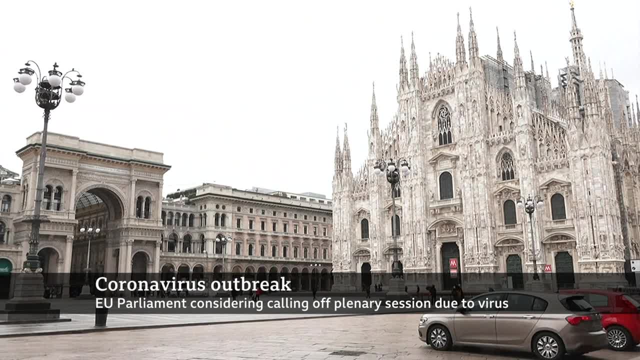 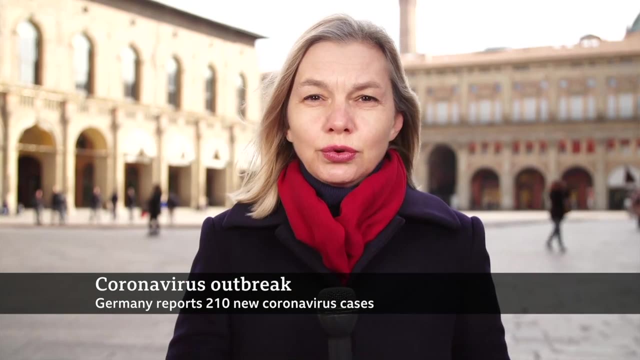 city like Milan. but what about the health care system? what concerns are people expressing today about whether or not it will be able to cope well? the hospitals at the center of this outbreak so far say they're really struggling, and this is in Italy's developed north. people have said that there are in 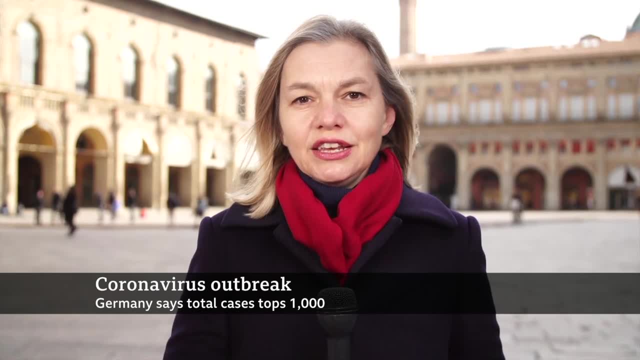 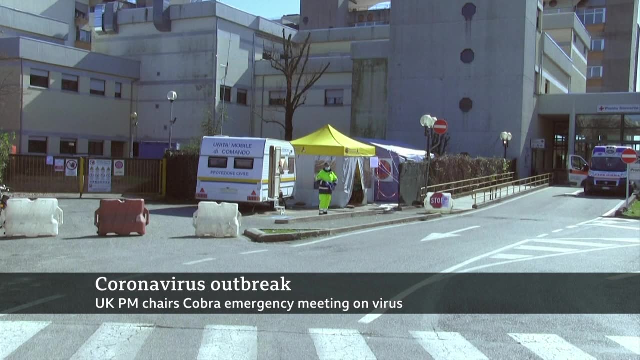 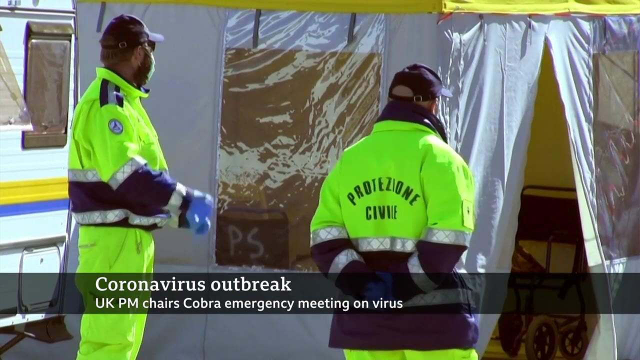 certain hospitals, they're having to set up intensive care units in corridors, and the fear is, if this virus spreads to southern regions where the health care system is perhaps not so good, then this could be a really, really difficult situation for the country as a whole, and really this is, I think, what is really. 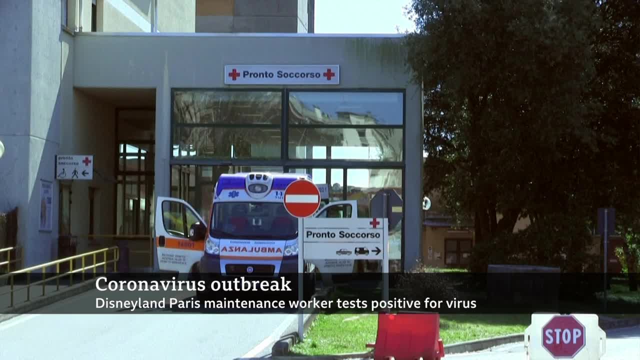 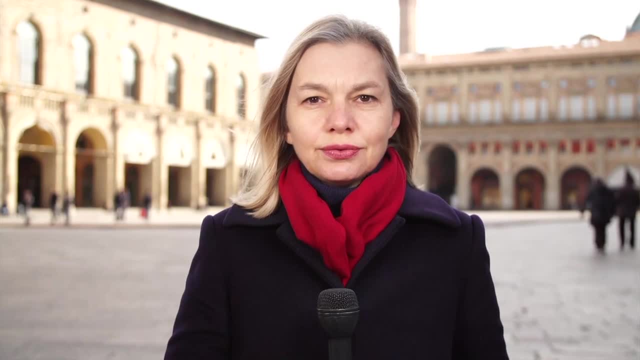 spooking people. I spoke to a couple of people yesterday and they were saying that inside the zone in Piacenza and they were saying that you hear the sound of ambulances all the time. it's really worrying people here. you want to the cruise liner which has been quarantined off the coast of California. 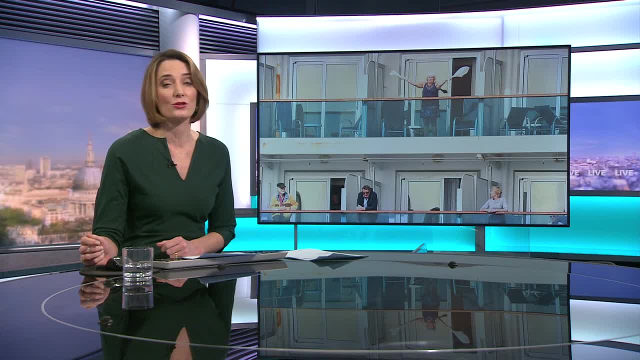 since an outbreak of coronavirus on board last Wednesday. it is due to dock at Oakland, near San Francisco. the passengers are expected to begin disembarking shortly, with the sickest being allowed off first. Sophie long as in San Francisco for us well, and what the governor of California called an. 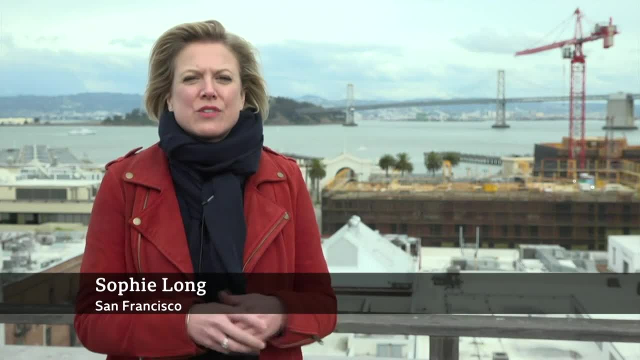 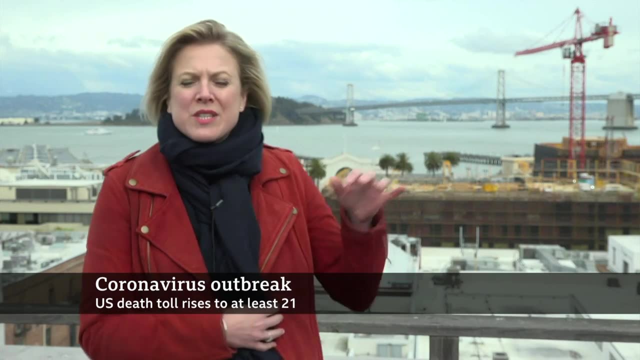 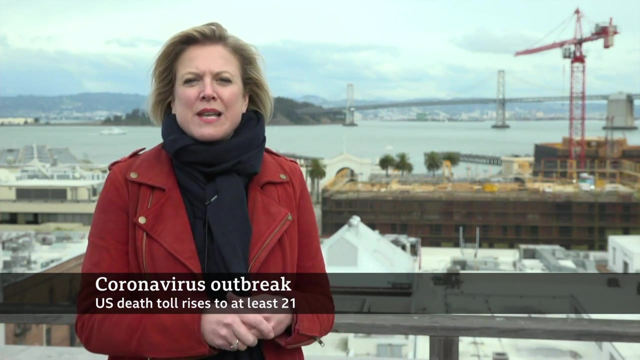 enormously complex operation. we now know that the Grand Princess cruise liner will dock at Oakland port at some point on Monday. now that's the port just across the water there I'm on the San Francisco side. it is a commercial but non passenger port. he couldn't give an exact time. he said that was dependent on cross currents and 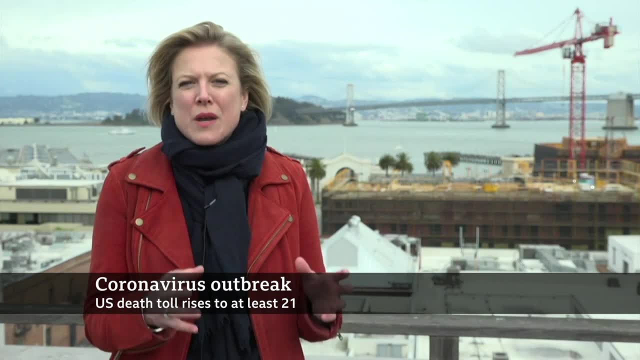 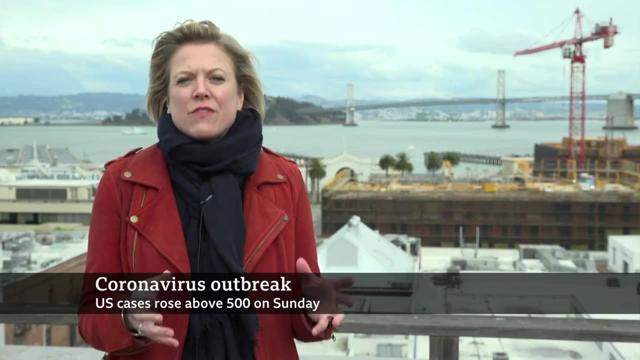 tides, but he is confident that that will happen at some point on Monday. then the disembarkment process will begin. the first people to be taken off the ship will be those in acute need of hospitalization. the next priority will be Californians. there are about a thousand people from California on board.